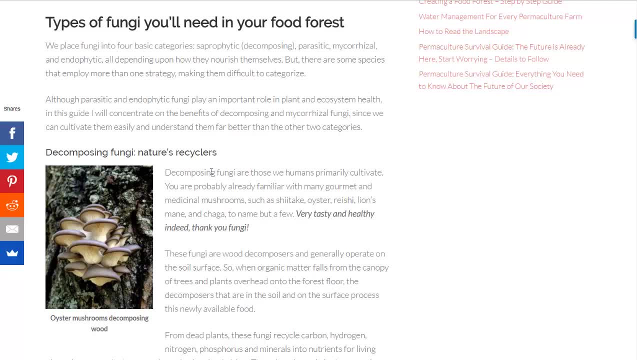 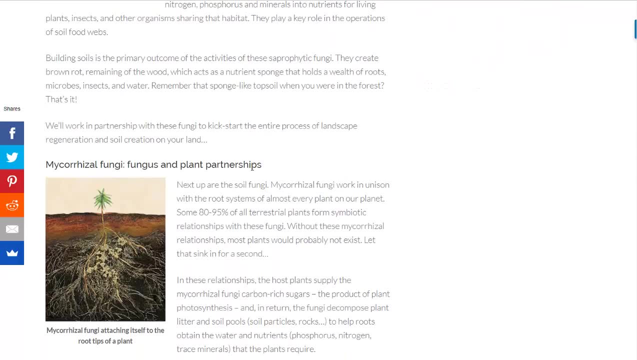 material, but they also act parasitically and can spread to different trees. But it's native in many parts of the world so it's not exactly considered an invasive species. Mycorrhizal fungi is fungi that lives in the soil and has beneficial relationships with plants. They estimate 80 to 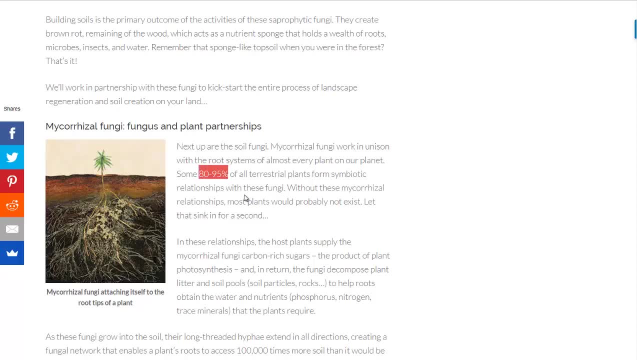 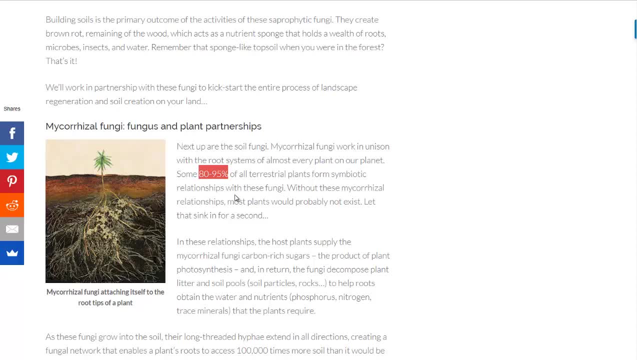 which ones don't? Some people say maple trees don't. Some people say they do, But mycorrhizal fungi. examples of those would be the boletes, the king bolete, or porcini mushroom, the morel mushroom. Morels and porcinis are kind of hard to cultivate for a fruiting mass, but mycelium could. 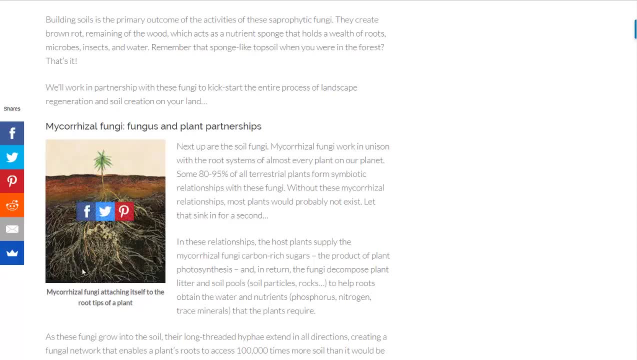 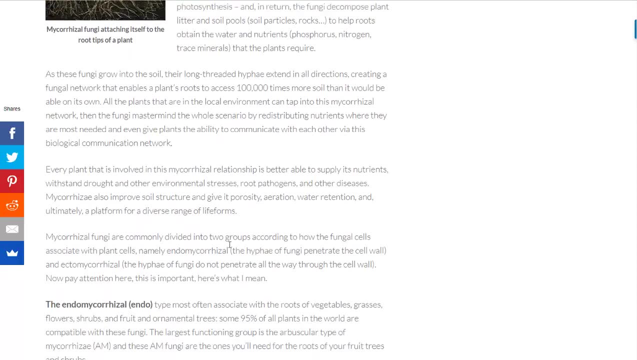 still create hyphae, which are the roots, the thin white hairs, and still populate the soil. But there's lots of different types of mycorrhizal fungi- I'm sure I'm mispronouncing that: The endo and the ecto. Now the endo is most likely associated. 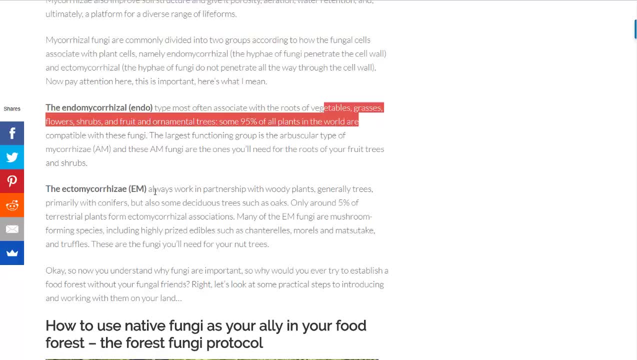 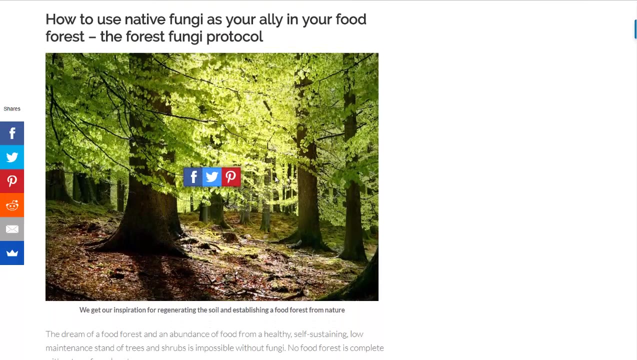 with the roots of vegetables and grasses, and they also talk about fruit trees And the ecto for nut trees and bigger trees. oaks are pretty much all types of woody plant material, And you want to have a little bit of both in the soil as well as the soil bacteria. So how do you do that? Well, 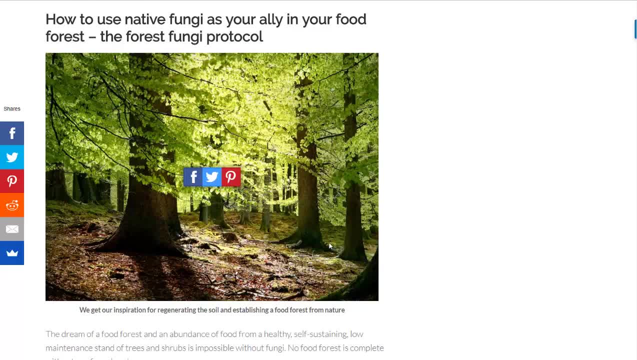 find some old growth forests in your area. Go out there and harvest some mushrooms that you start seeing out of the ground around trees that are similar to the ones you're trying to grow. You know, wild fruit trees if you're growing fruit trees. wild nut trees if you're growing nut trees. 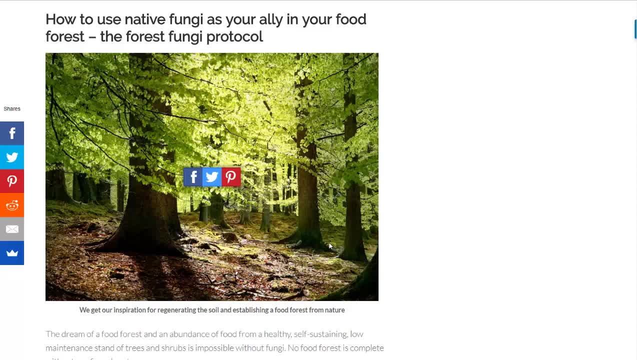 that sort of thing. And you can take fruiting mushrooms, take the mycelium or I'm sorry, but take the spores off of them by making a spore print and then propagating those spores all across there using a compost tea-like mixture- And we'll get into that in a second. 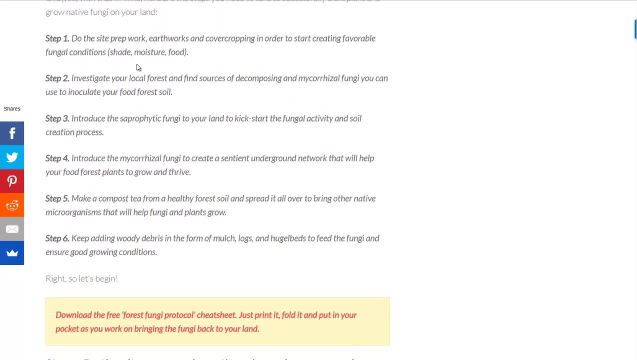 They talk about these six steps. Do site prep work, So make sure you create an environment that's capable of supporting fungal life: Good shade, moisture and food, which is woody debris. Chopped up leaves and grasses will also work to a certain extent, but mushrooms really love wood.